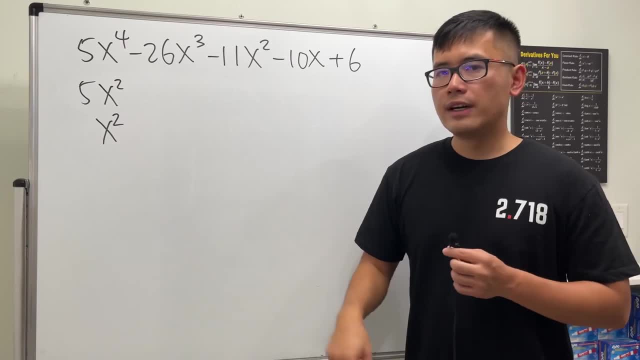 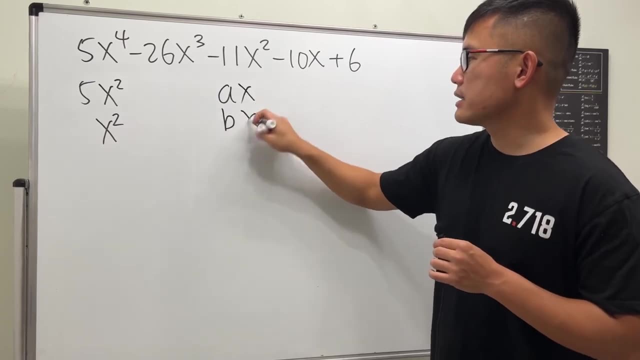 You cannot just look at negative 11 and say 1 and negative 11, or negative 1 and 11, no, Right, here we can only put down some number a times x and then b times x, Because when you multiply this and that this is not the only way to produce the x squared term. 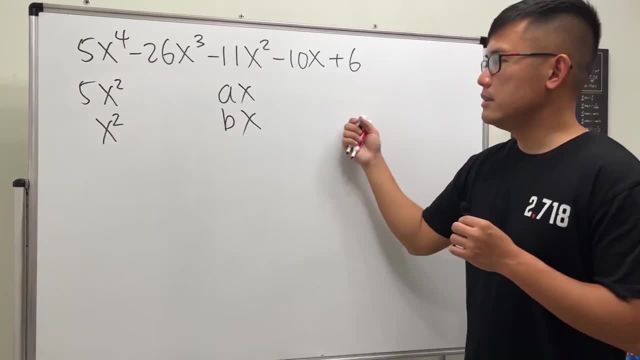 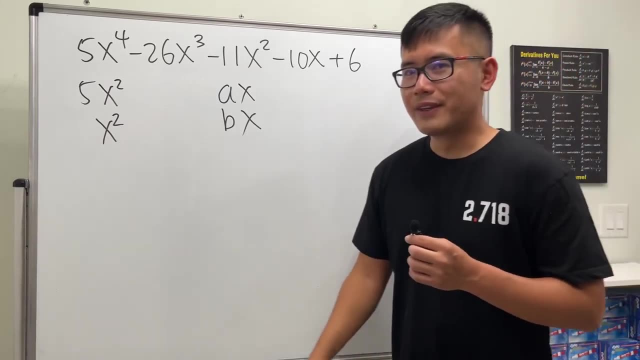 We will also have to consider the 5x squared times constant here, right? So we really have to put down a and b, right here. And what do we do next, though? Well, here, this is the first time- we are using the cross method or the tic-tac-toe method. We do this times that which we can get, 5bx to the 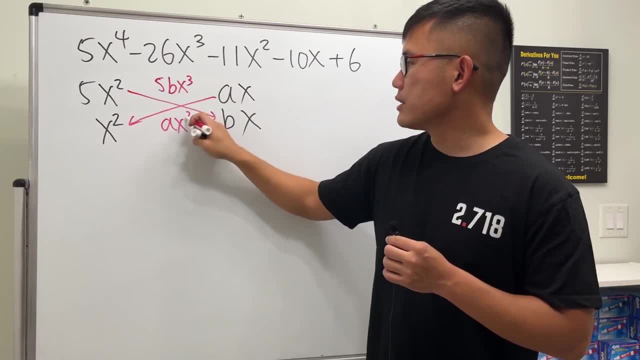 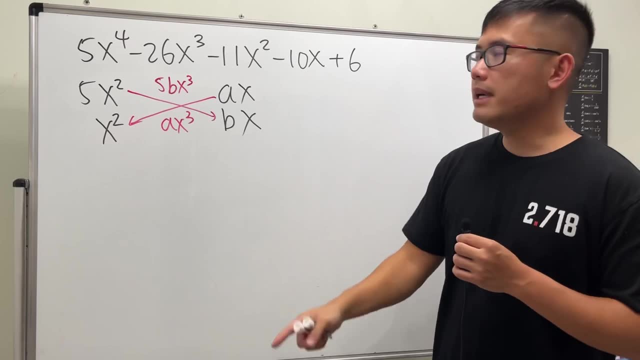 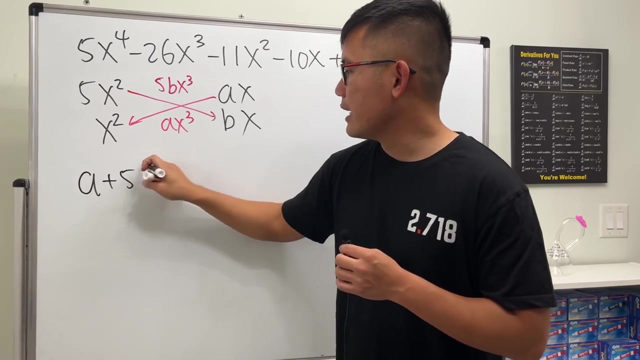 third power, and we do this times that we get ax to the third power. These are the only two ways to get the x to the third power term. all right, So that means we must have this coefficient plus that coefficient equals that coefficient which we know we must have. a plus 5b equals negative 26.. 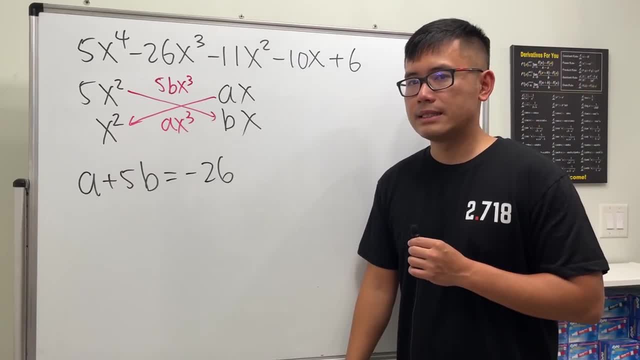 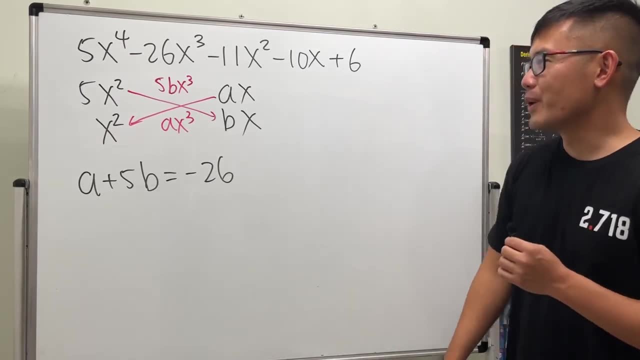 Yes, we are going to solve a system of equations, But anyway, come here Now we have 6.. This is crazy. We are just going to break it apart and then it really depends on where we put it right. So let's just hope for the best. I will say: This is not easy. all right, So let's just go ahead and 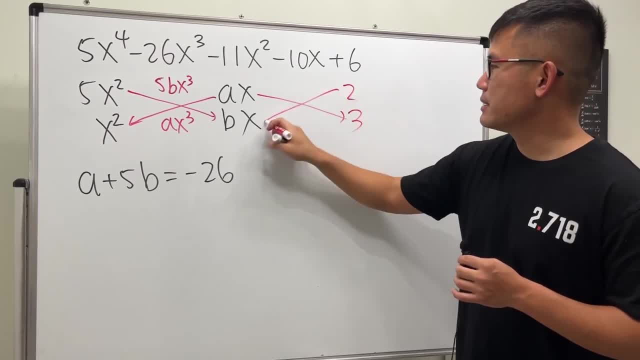 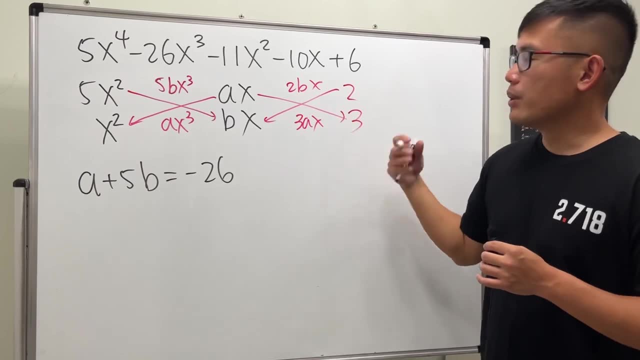 try 2 and 3, and let's do this times this, this times this, and we will get 2bx and this times that is 3ax. So same idea. These are the only two ways to produce the x term, So we must have this. 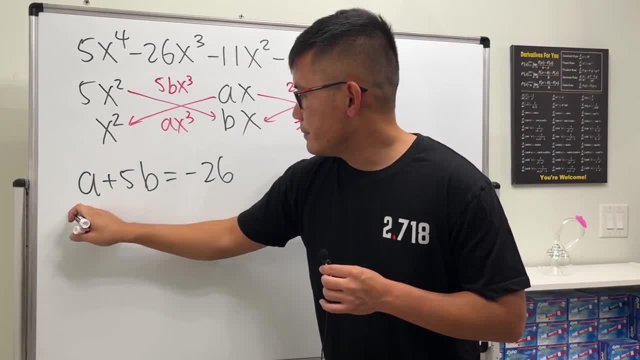 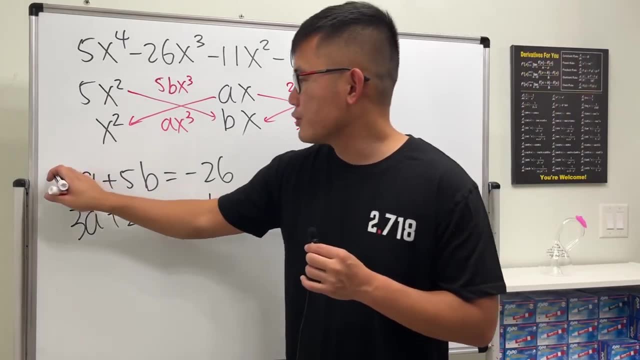 plus that equals that. So we have 3a plus 2b equals negative 10. And the reason I put this down in red is because I am not sure if they will work or not. And now let's just go ahead and solve. 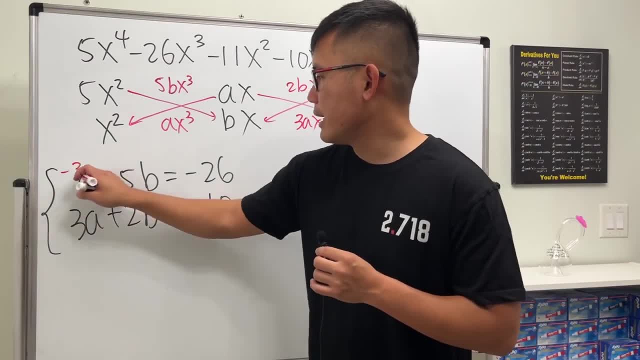 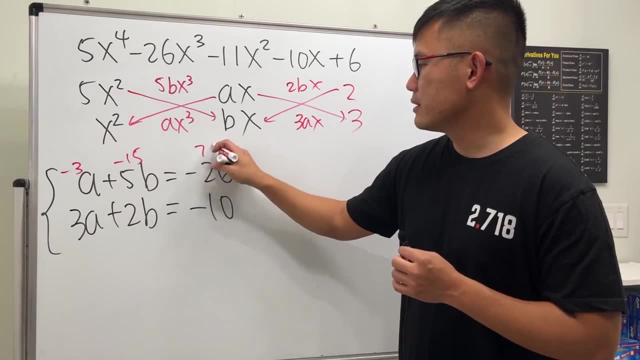 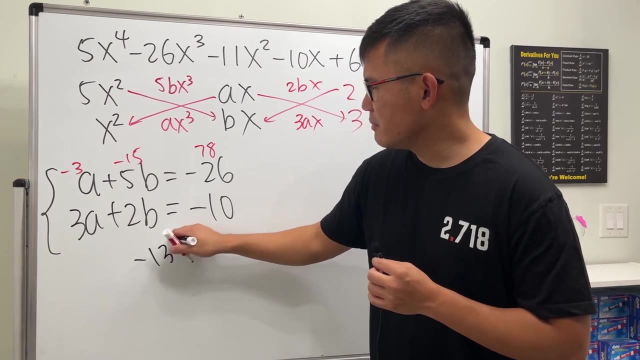 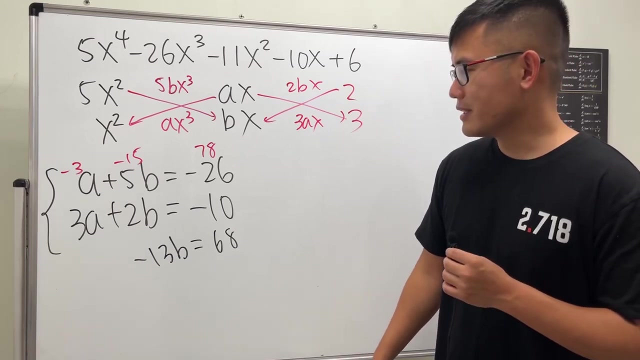 this real quick, So perhaps I'm just going to multiply everybody by negative 3. So this is negative 15. And negative 3 times this, that's a pretty big number. Cancel And then we have negative 13b equals 68. I don't think this works because actually I've told you guys that the 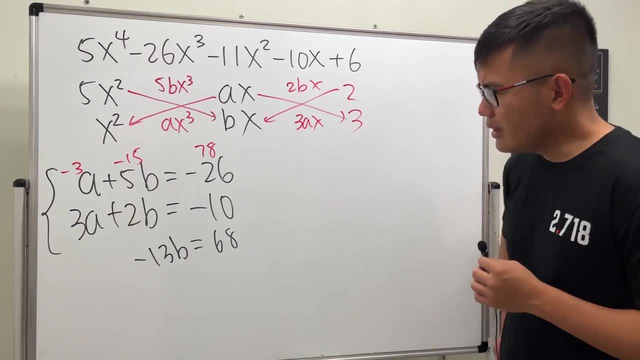 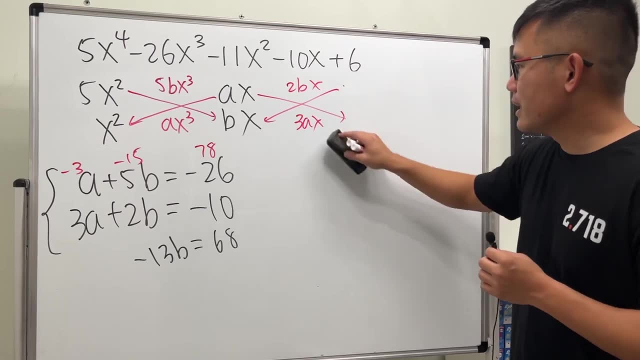 coefficients are integers. If we don't end up with an integer, then we eh. no good, Let's just try another one. So maybe I just put down the wrong order And, of course, in order to make this fair, I will have to say: 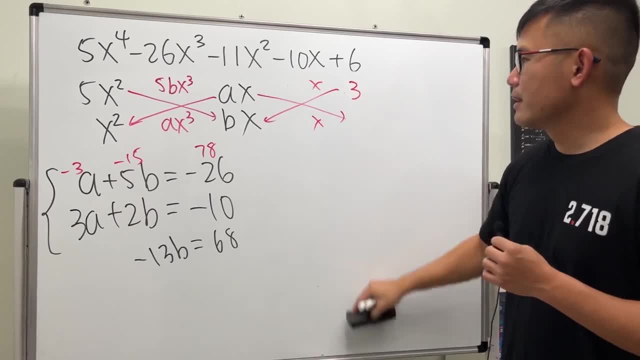 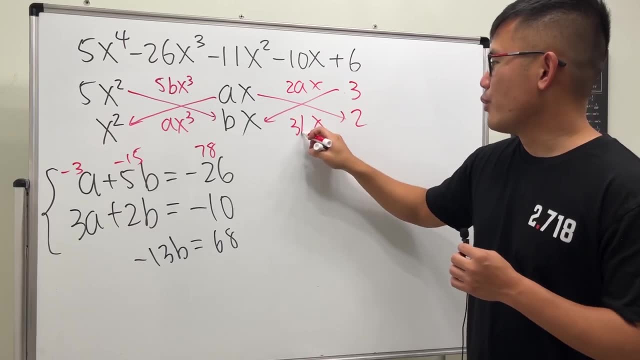 hey, they can all be factored in terms of a quadratic times a quadratic and then all integers, right? So that's how we can make it more fair, But we will continue here. So this right here is 2a plus 3b. 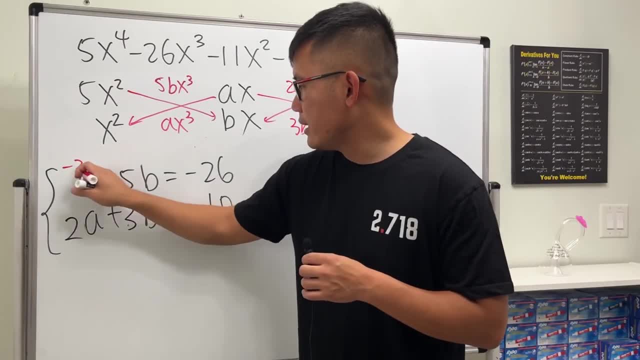 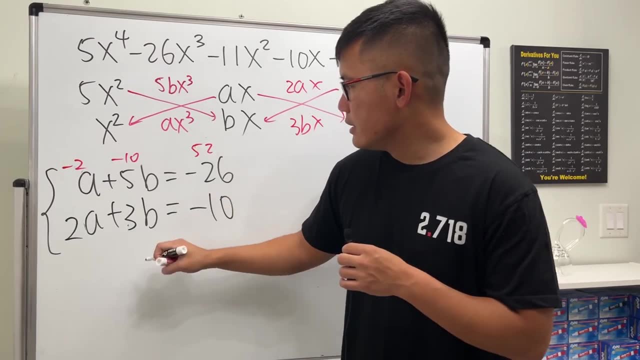 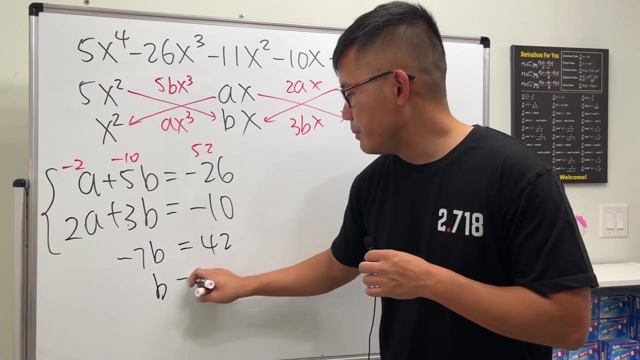 All right, let's try this again And we'll multiply everybody by negative 2. And that will be positive 52.. Yes, Combined this is going to be negative. 7b equals 42. So b could be equal to negative 6.. And if b is equal to negative 6, put it here: that's negative 30.. 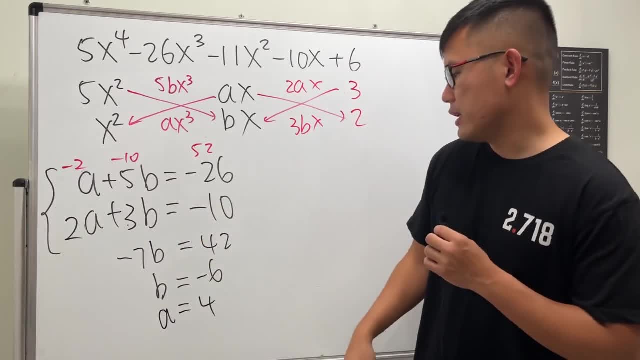 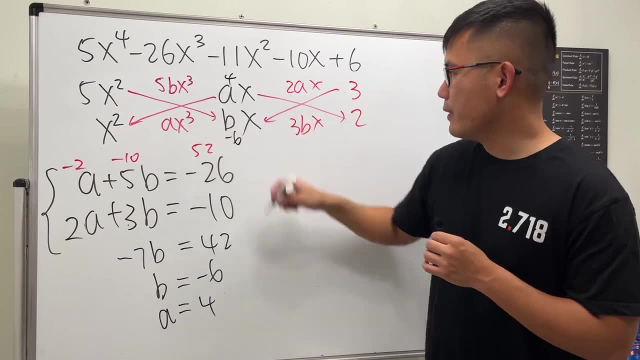 So that means a has to be equal to 4.. Just do this in your head, right, Okay? So right now we are saying that this is negative 6 and this is 4.. And what I will do is I will just multiply this. 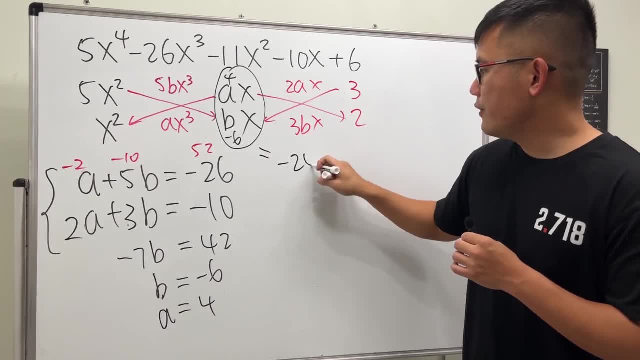 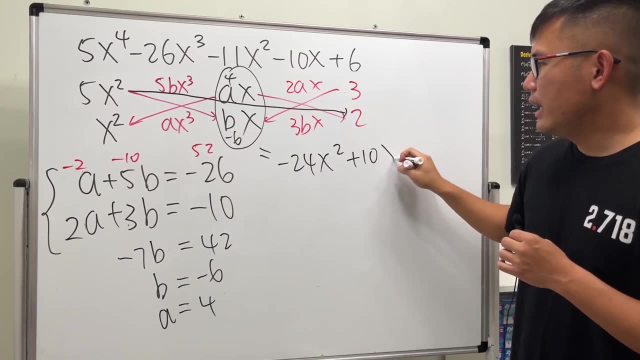 and that which I will get negative 24x squared, And then we will have to do this times this That will give us plus 10x squared, And then take this times that That's plus 3a. It works. 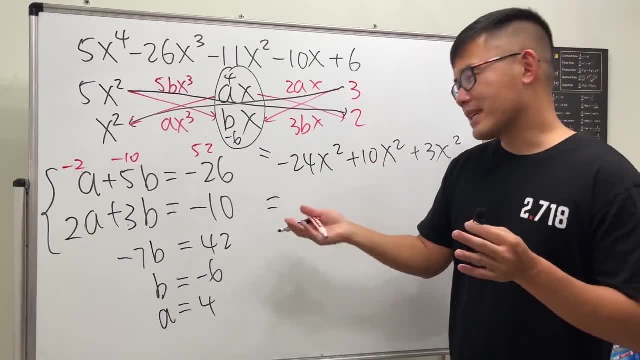 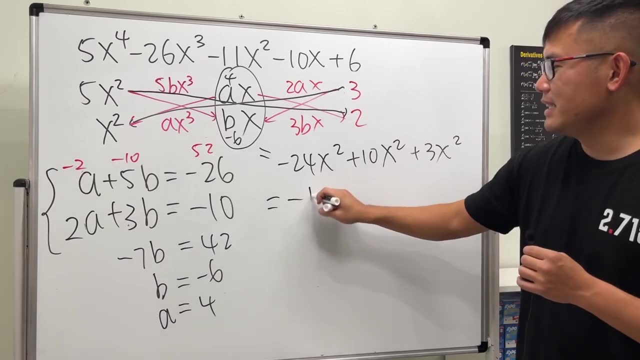 I didn't prepare this already, It's just I. well, I kind of did, but like I forgot my yeah anyway. Yeah, 13 plus this is negative 11x squared. We know? the answer is just this. 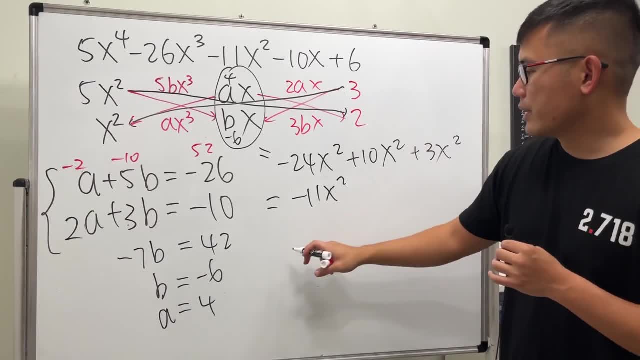 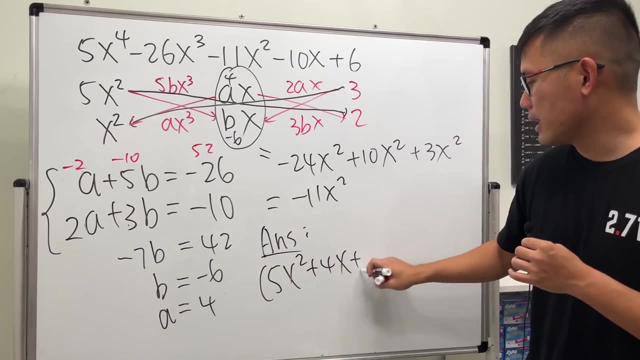 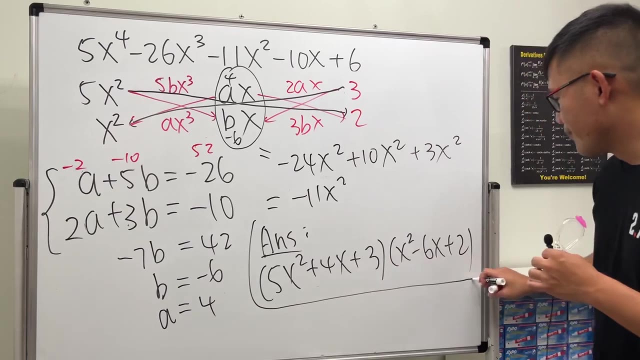 this that and this, this, that. So, ladies and gentlemen, this right here, I'll just say: the answer is equal to 5x squared plus 4x plus 3 times x squared minus 6x plus 2.. Yeah, cool, All right.